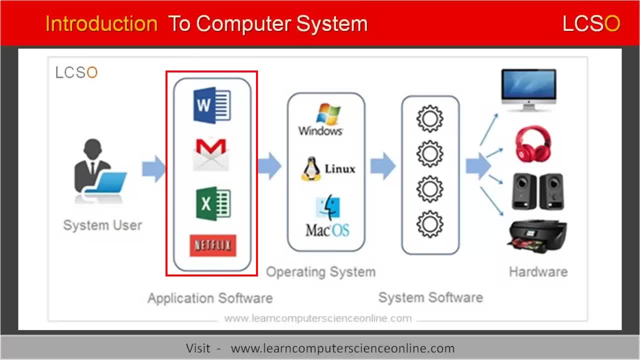 Such as Microsoft, ward and PowerPoint, Whereas the system software is a special type of software that is internally used by the computer itself to manage and operate the various components- hardware components connected to the system. The operating system is the most. 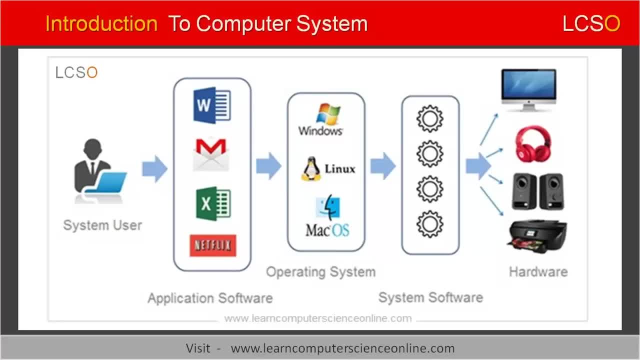 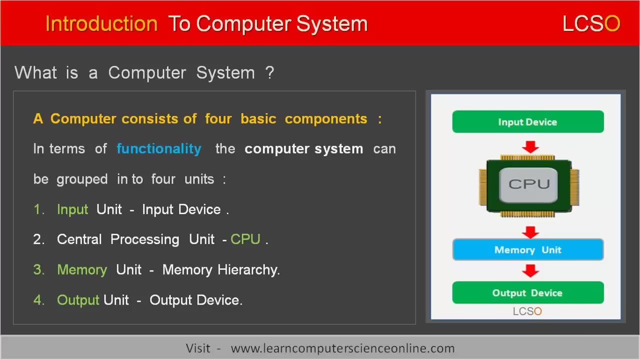 important system software used by the computer. The operating system basically provides an interface to the user to interact with the system. Let us now understand the architecture of the computer system in terms of the functional units. The entire functioning of the computer can be grouped into. 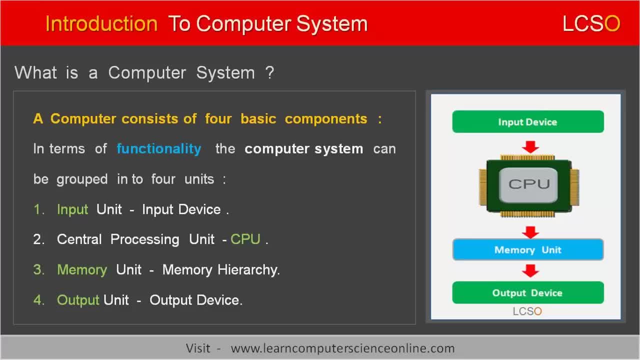 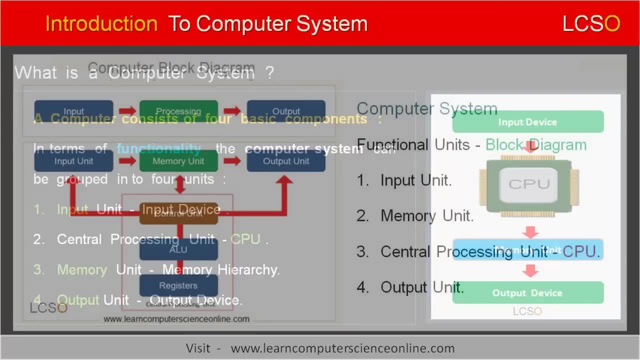 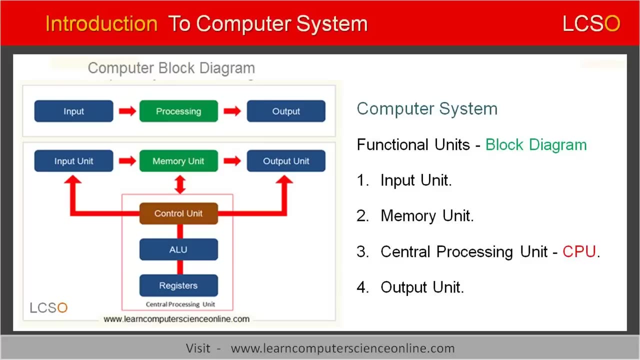 various functional units. Let us understand some important functional units of the computer system with the help of a computer block diagram. The computer system working can be grouped into four major units. Each unit performs a specific function in the working of a computer. The four major units of the computer units: 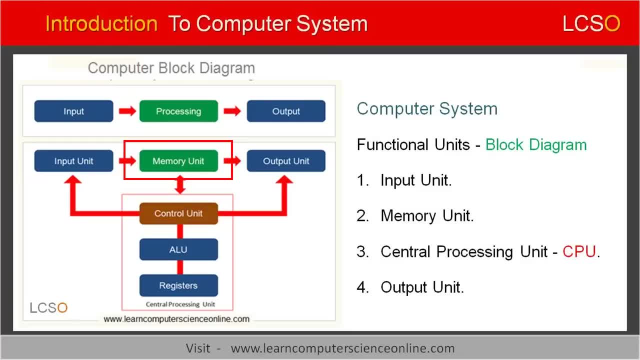 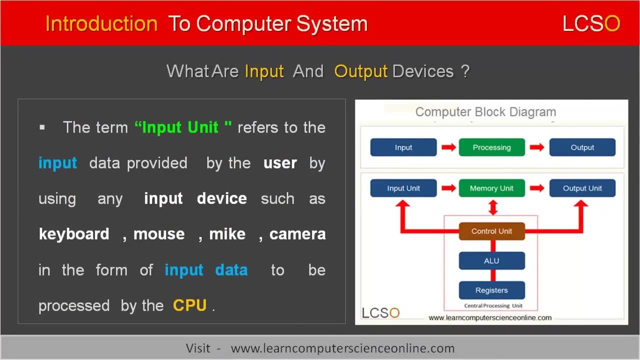 are: first, input unit, second, memory unit. third, central processing unit, also commonly referred to as CPU, and the fourth unit is called output unit. The input unit consists of various input devices connected to the computer system, such as keyboard, mouse, scanner. The main function. 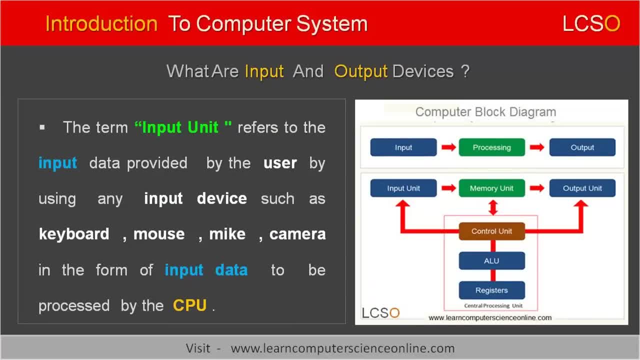 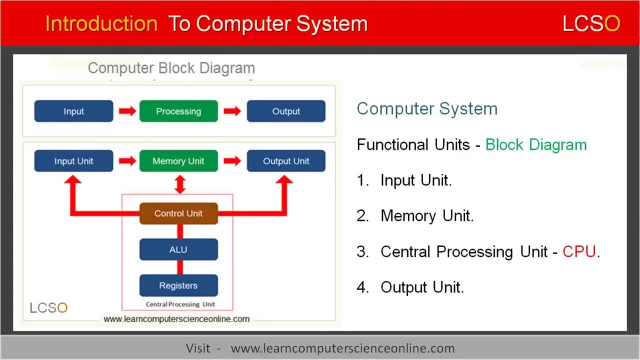 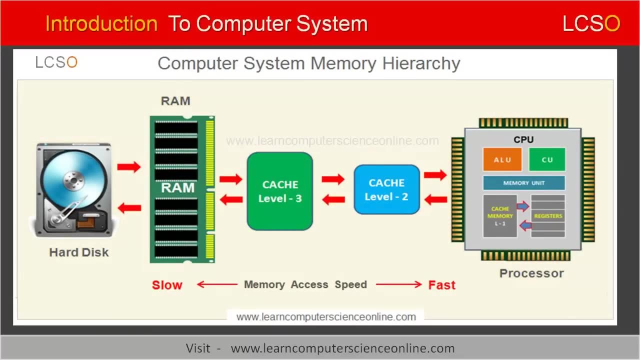 of the input unit is to accept the data received from the input devices. The next unit is called memory unit. The computer memory unit consists of different types of memories used to store the data and the program instructions during the program execution. The computer uses different types of memories, such as disk memory, random. 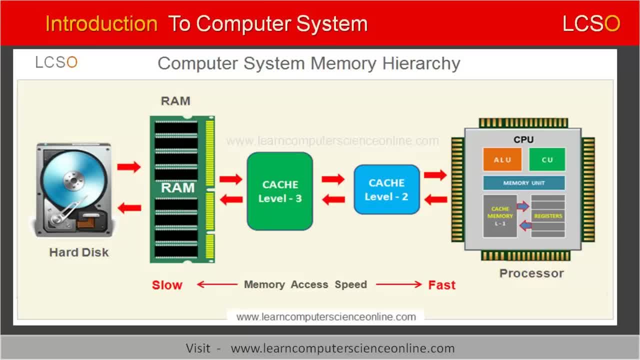 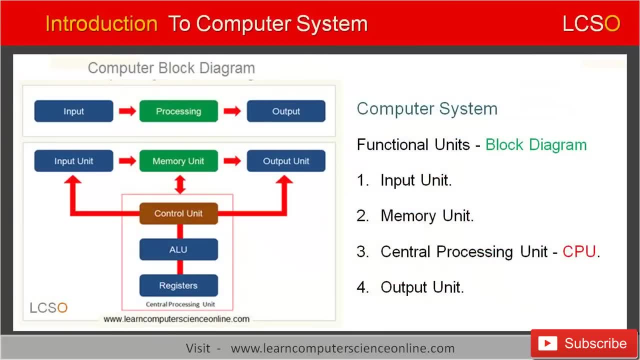 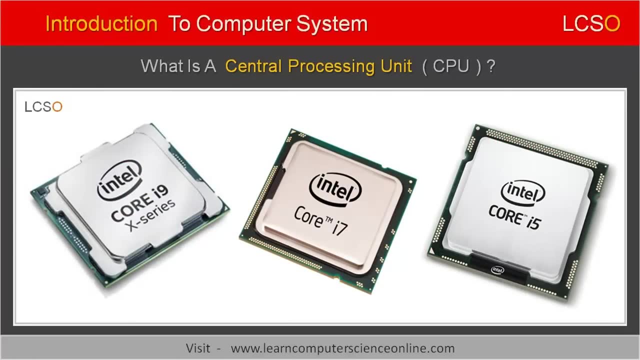 access memory called RAM, cache memory, and the CPU memory registers. The next unit of the computer is called the central processing unit and it is abbreviated as CPU. The CPU is also commonly referred to as processor or a microprocessor. The CPU is the brain of 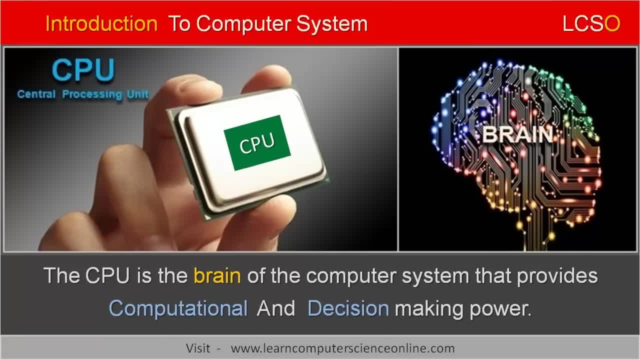 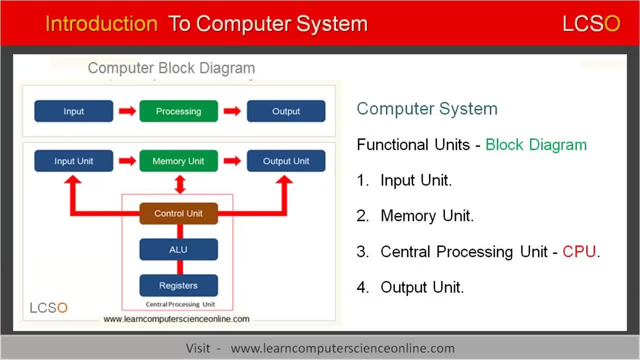 the computer and provides the processing power to the computer system. The main function of the CPU is to execute the computer program. The fourth unit of the computer is called the output unit. The output unit consists of various output devices connected to the computer system, such as display, monitor, printer, projector and other. 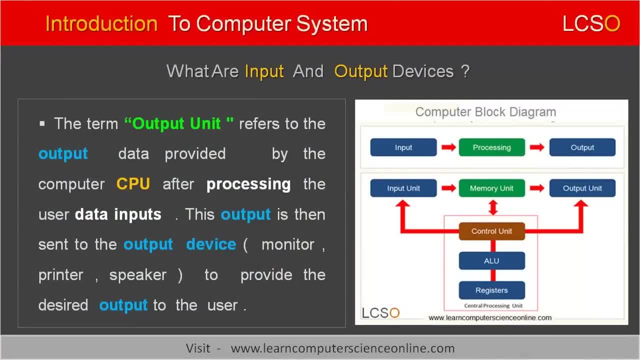 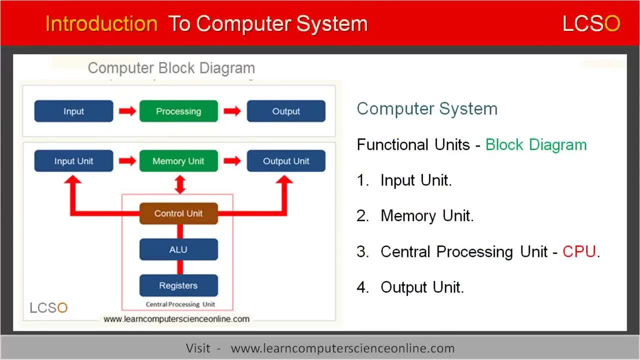 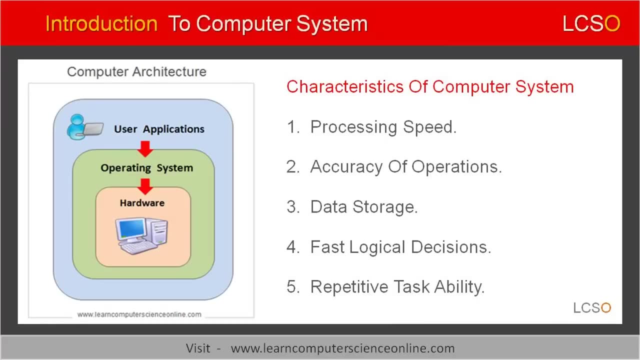 output devices. The main function of the output unit is to present the processed data by the computer. all right, So far we have discussed various functional units of the computer. Let us now move on to the next topic, that is, important characteristics of the computer system. 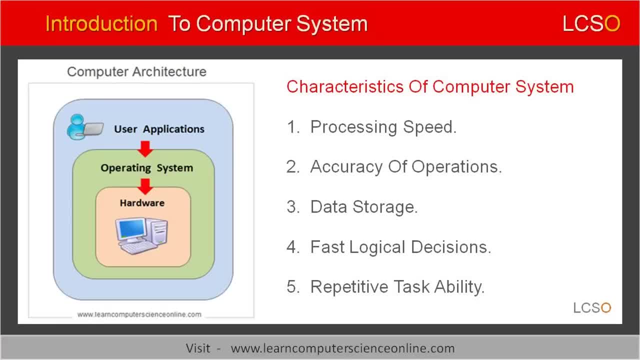 The computer system has four important characteristics. These characteristics are: first, speed, second, accuracy, third, storage, fourth, fast decisions and fifth, ability to perform repeated tasks. The computer can operate at very high speed. The computers can also operate with remarkable accuracy, without any mistake. 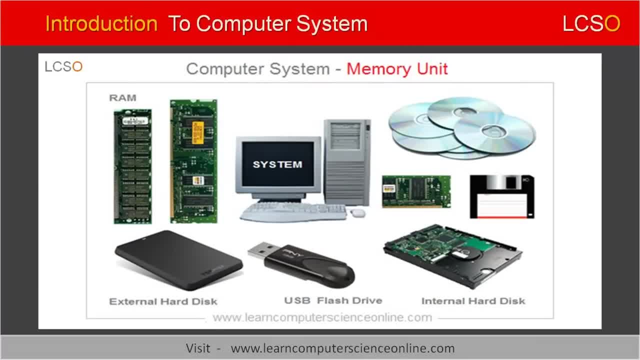 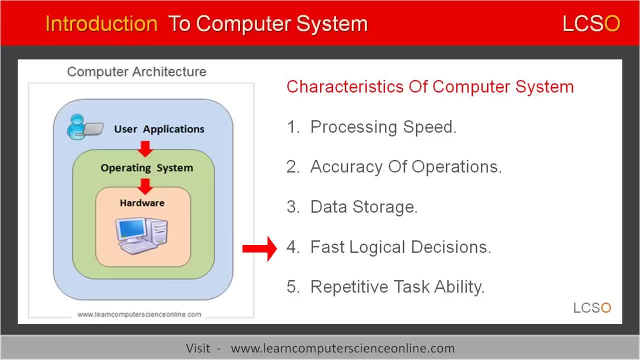 The computer also provides different types of storage devices to store the large volumes of data. The processor inside the computer is designed to take fast decisions as per the program instructions. Similarly, the computer can work continuously and repetitively perform the programmed operations without any break. 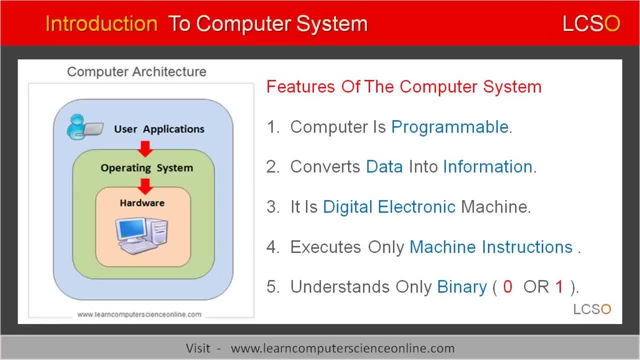 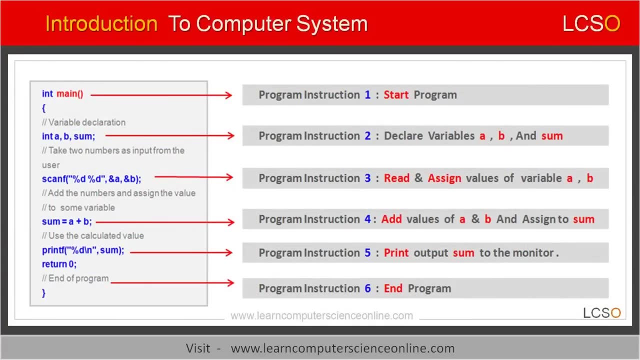 Let us now move on to the next topic, that is, important features of the computer system. The computer system has some important features. These features are: first: the computer is a programmable. The term programmable means each task performed by the computer is directed by the set of. 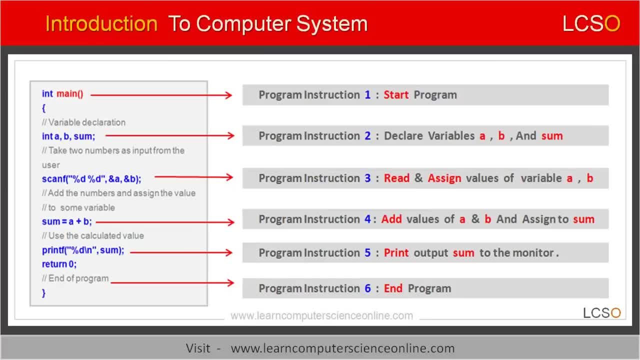 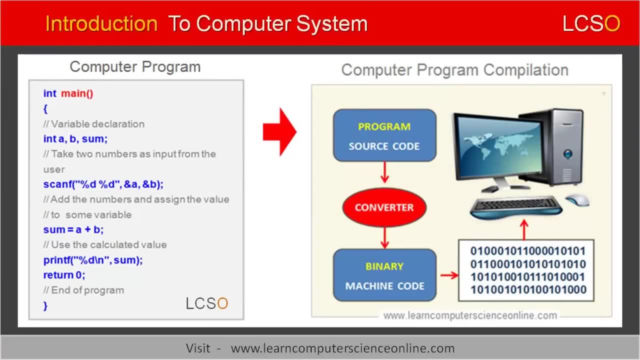 instructions. This set of instructions is called as a computer program. The computer program directs the computer system to perform specific operations. In other words, the computer will perform the task only as per the program instructions. Second, the computer is used to process the data, The data processing. 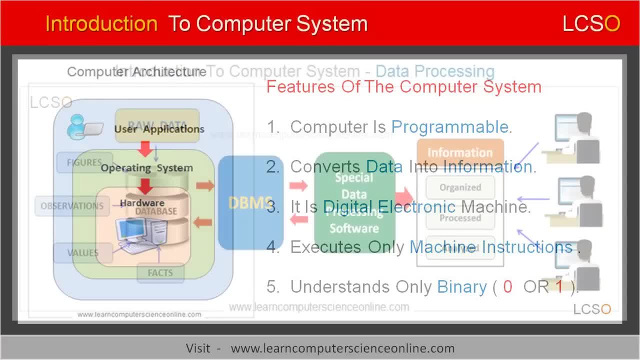 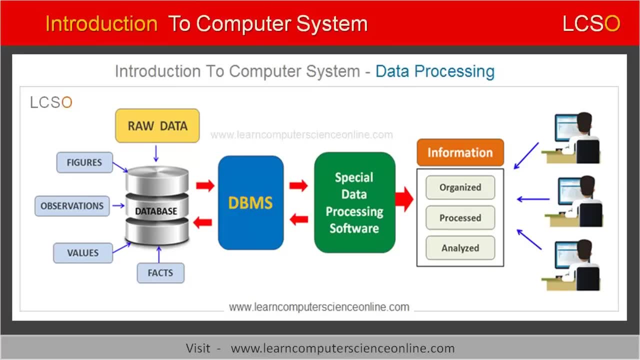 is one of the most common use of the computers. The computer process the raw data and produces the information. The data cannot be meaningfully used in the raw form. The raw data needs to be first converted to processed data so that it can be used for some meaningful work. 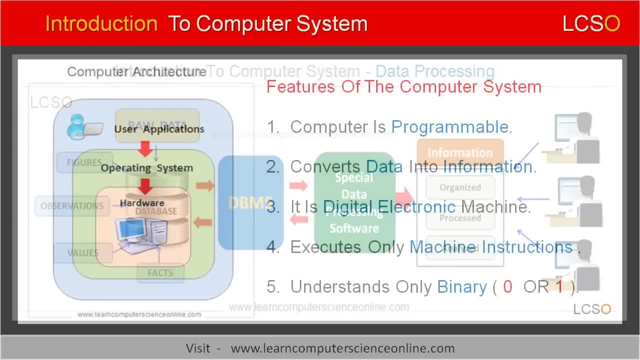 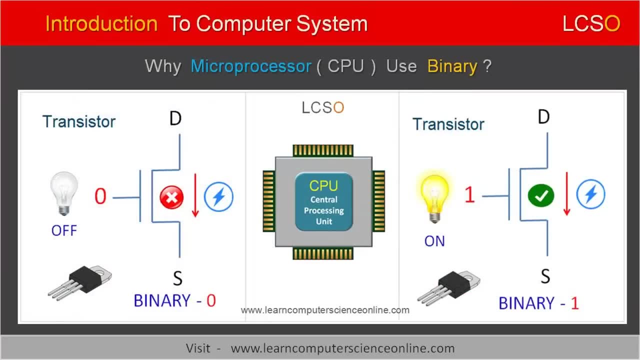 such as decision making within an organization. Third, the computer is digital electronic machine. The computer is called a digital electronic machine because it contains electronic components and computer needs an electric current to operate. The term digital simply means the computer understands the language of only. 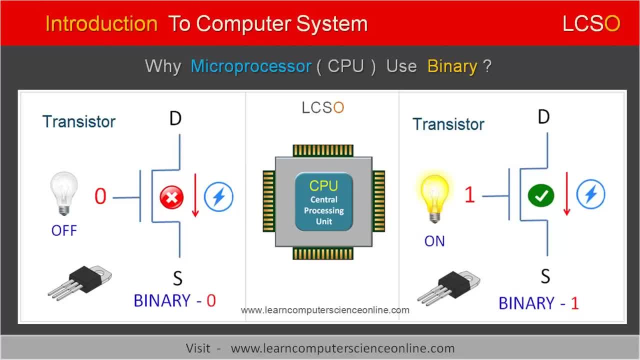 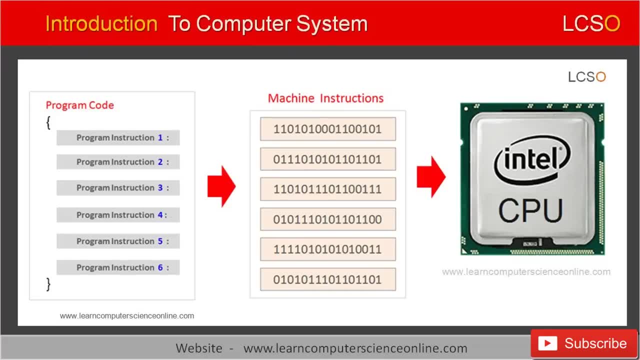 0 and 1, called the binary number system. The computer can understand and execute instructions written only in binary. These instructions are called machine instructions. The machine instructions in binary consist of only two numeric numbers, that is, either 0 or 1. The CPU can 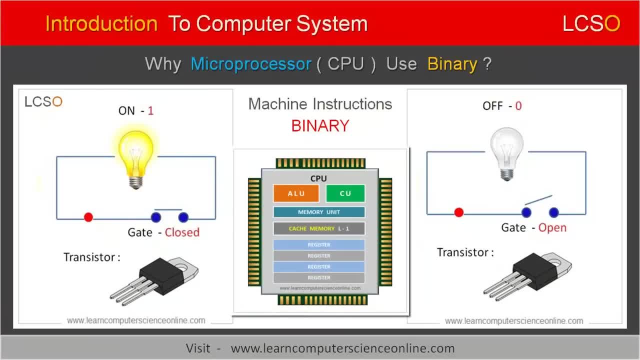 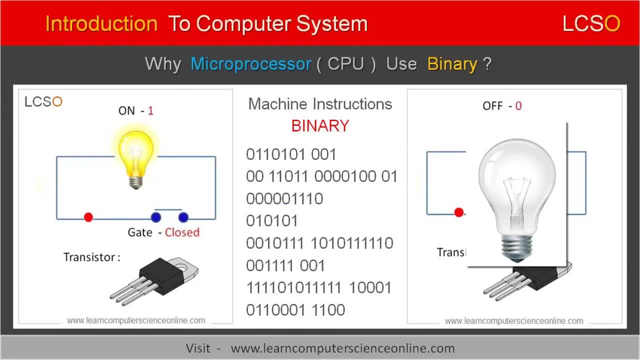 execute the program instructions encoded in machine language. The machine instructions consist of sequence of only two numeric numbers, that is, either 0 or 1. The binary code is also referred to as machine code or machine language. The computer's microprocessor works as a brain. 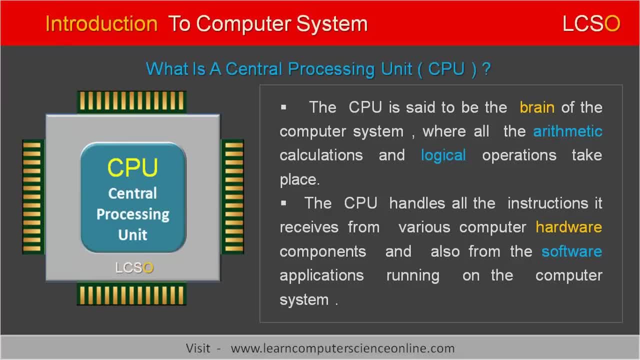 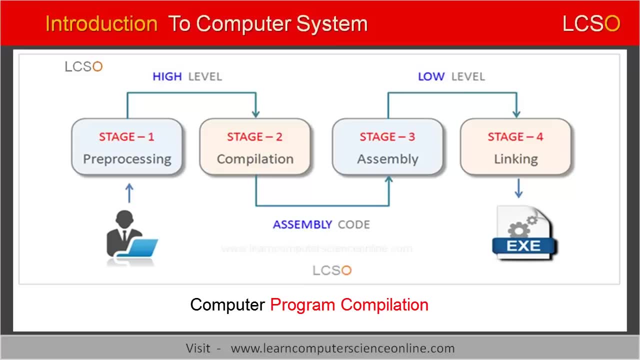 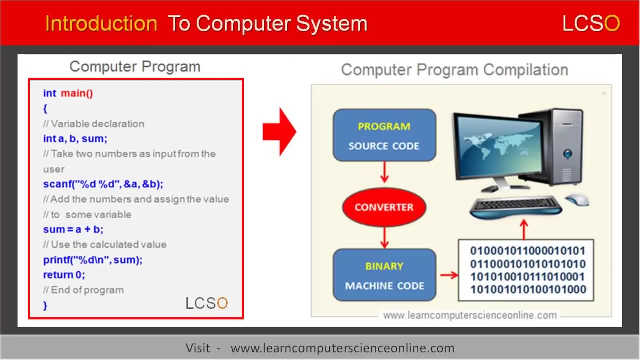 The processor performs all the arithmetic calculations and also handles the logical operations. The program compilation is another important fundamental concept related to the computer that you should be aware of. The computer programs are written using any high level, human readable programming language, such as C language, Java and Python. 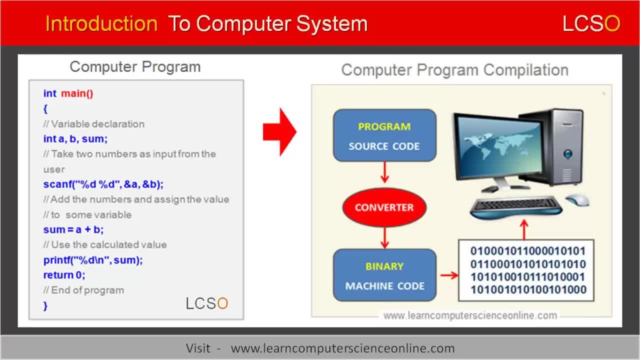 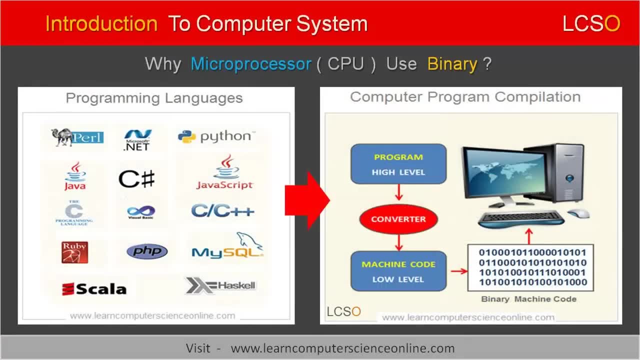 However, the computer processor can decode and execute instructions only in machine code in binary. So it doesn't really matter in which high level programming language you write the program code, because eventually all high level computer programs must be first converted to low level machine code in binary that CPU can directly execute.